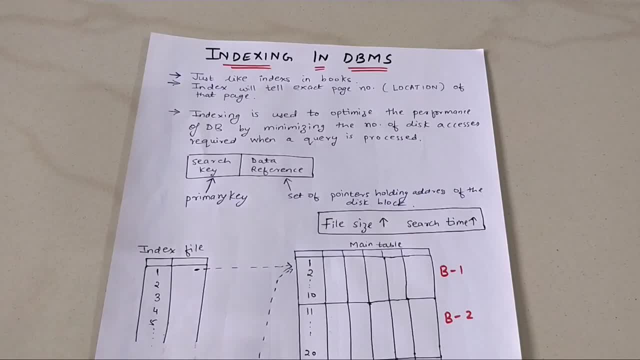 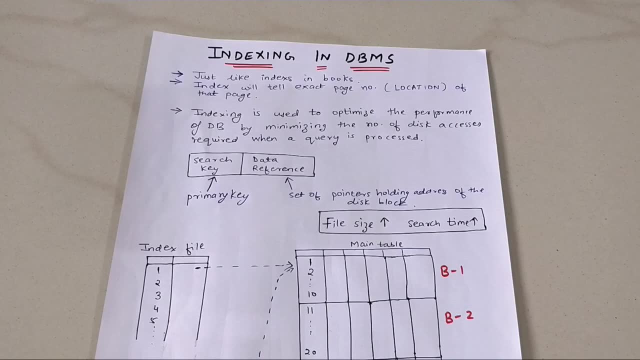 hello everyone. welcome back to my channel. in this video, we are going to study about indexing in DBMS. now, indexing in DBMS is just like indexes in your any book. so so why is an index used, even in your books? why is it used? it is used so that you take less time to reach a particular page. so, as I've 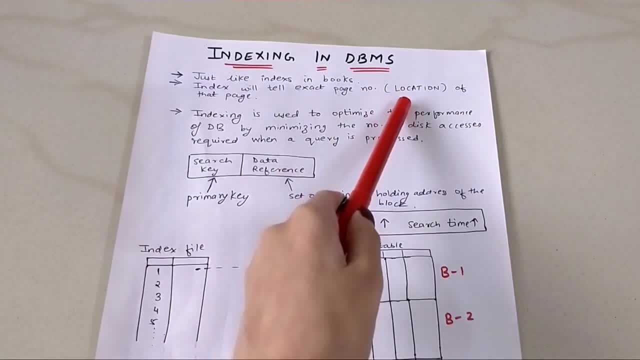 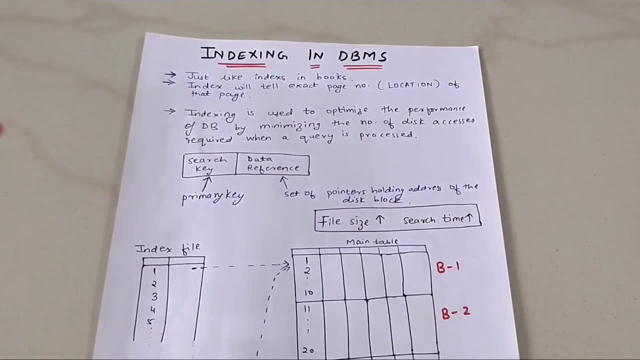 written over your index will tell exact page number, basically location of that particular page. so similar thing, similar thing. similar concept is in indexing in DBMS as well. so now if I, if you have a book, now if I tell you, and if you didn't, if your book does not have any index and if I tell you, go and find. 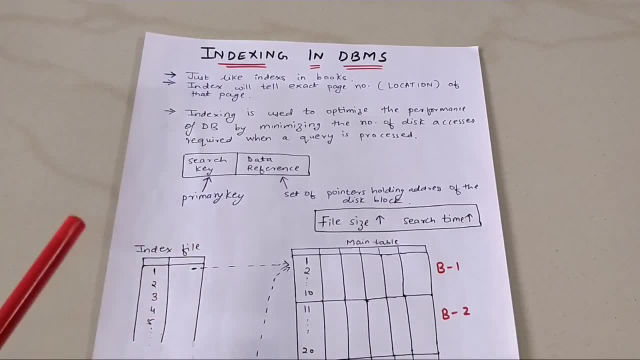 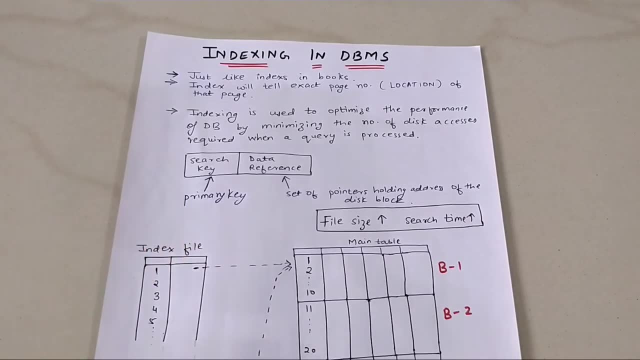 a page where the data about so-and-so, for example the page where alpha beta pruning is given. go and find that particular page where alpha beta pruning is written over. the information about it is written so and there is no index. what will you do? you will check each and every page one by one, and that is very time-consuming. 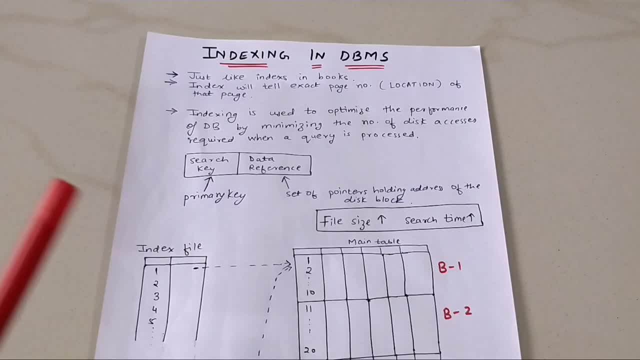 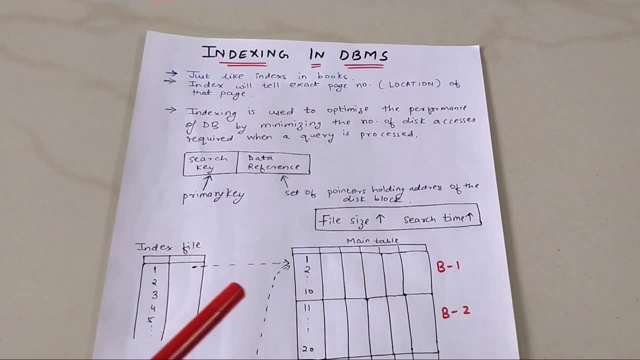 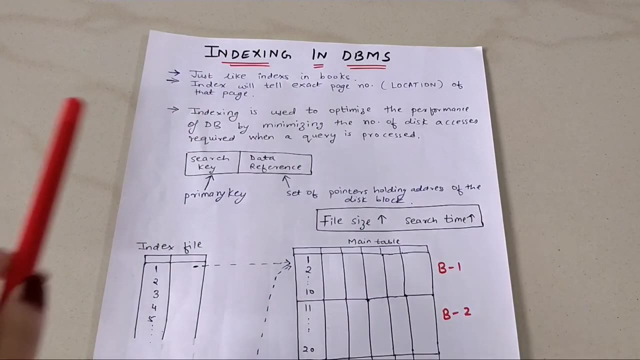 it will take a lot of time to find that particular page, but if you have an index in your book, what you can do is you can check the index and you will know exactly at what page number that particular topic is there. so you will already know. similar concept is applied in indexing in DBMS as well. indexing is 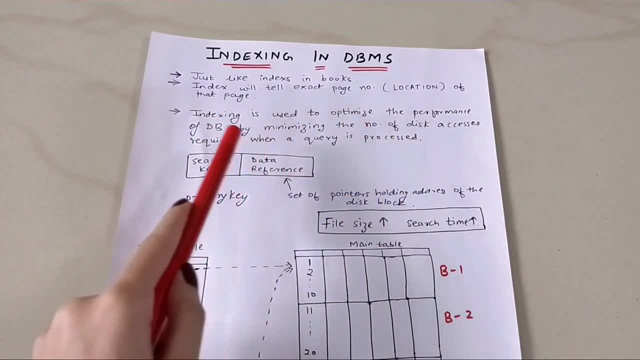 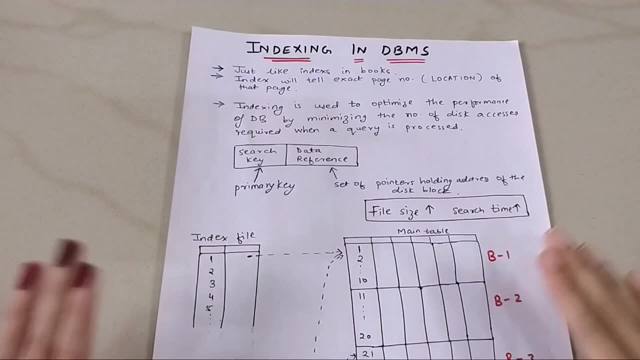 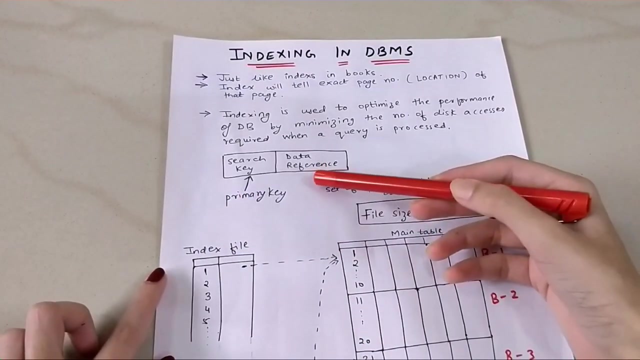 used to optimize the performance of DB by minimizing the number of this disk accesses required when a query is processed. you need to understand. there are two kind of tables considered over here. one is the index table, which will have only two columns. okay, this is a structure of a of an index table, so one. 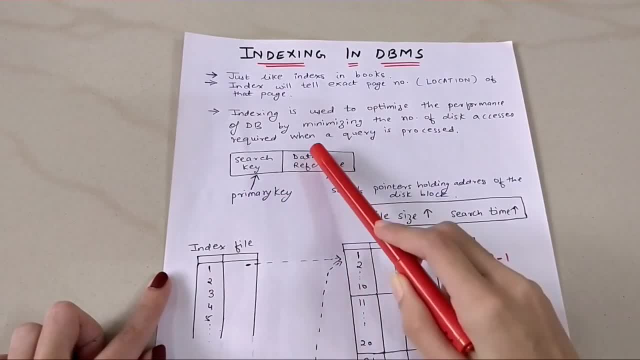 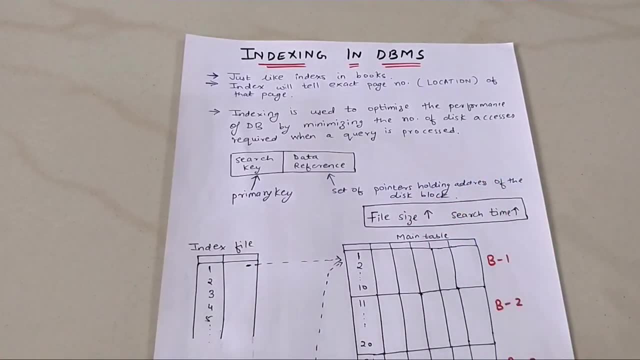 column will be the search key, basically your primary key, and the second column will be data reference, which is a set of pointers holding address of the disk. block now. what is block? now, as your books have pages, similarly, your tables will have blocks. now, as you have pages, similarly, your tables will have blocks. 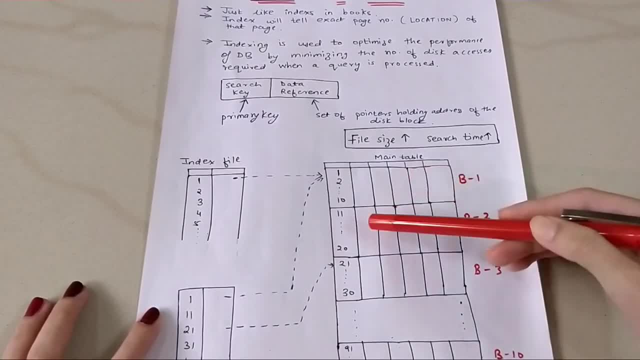 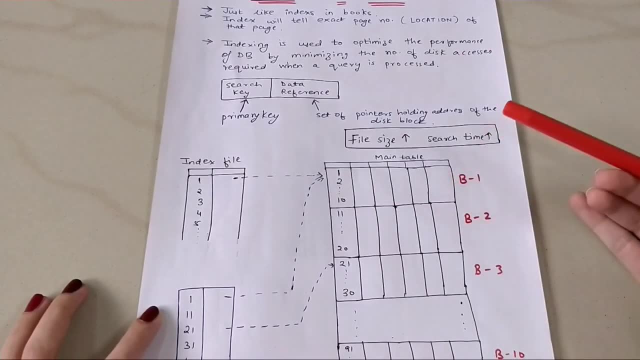 so, as you can see over here, this is your, this is your main table. the main table has many rows and it has many columns, many fields like, for example- let's consider: this is an employee table, so employee id, employee name, employee address, designation, manager and whatnot- salary, everything. 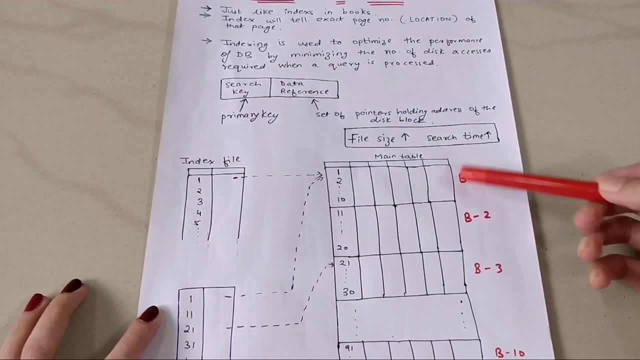 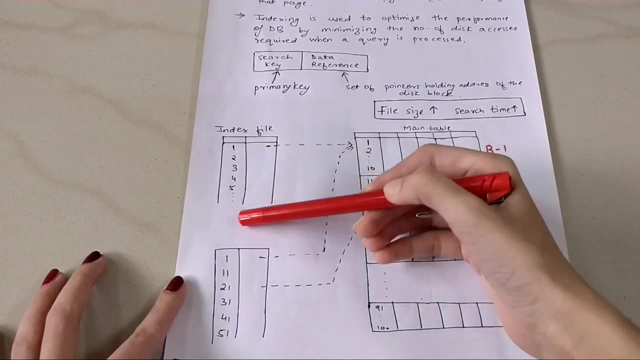 so it has a lot of rows and what? how is it categorized? so from employee 1 to 10, they are considered into block 1, 11 to 20, it is considered into block 2, and similarly we have 10 blocks over here. but my index file. now there can be different types of index file and there are three types of. 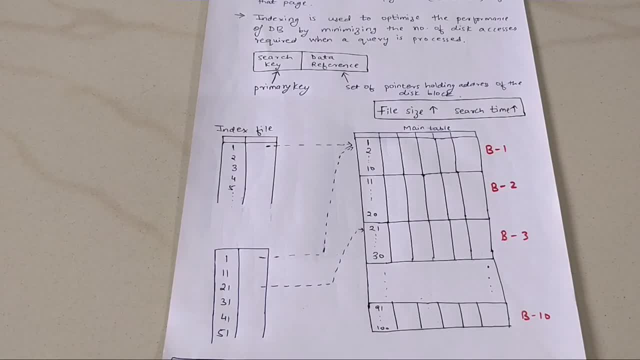 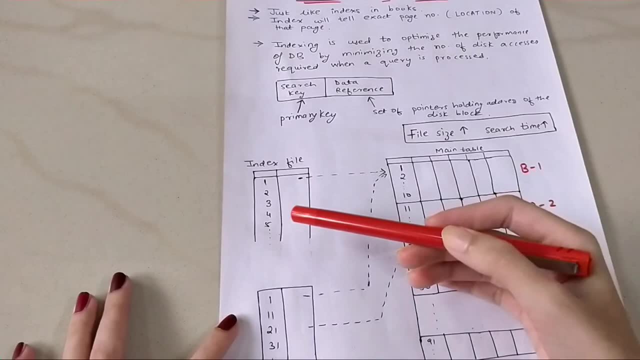 index file, which three types of indexing in dbms, which will be uh, which, which will be explained another video, but here i'll explain in short now, for example, this is your index file. here all the primary primary keys will be: will be written over one, two, three, four, five. 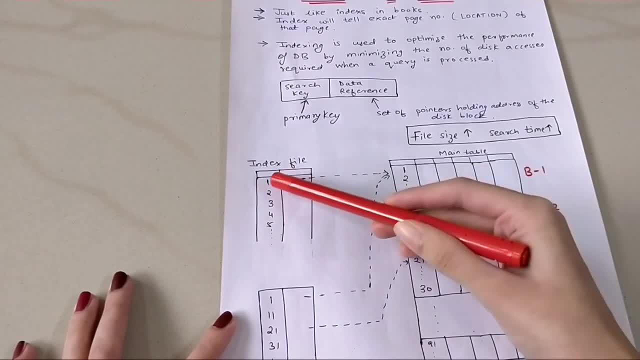 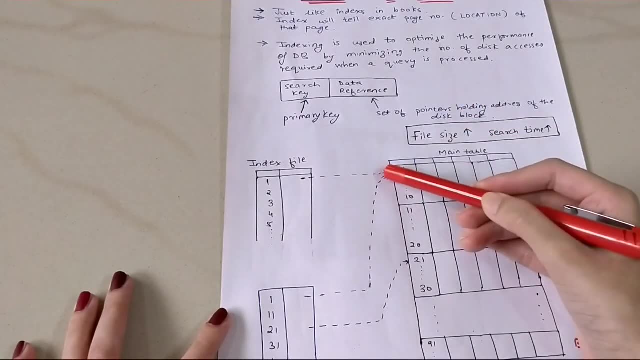 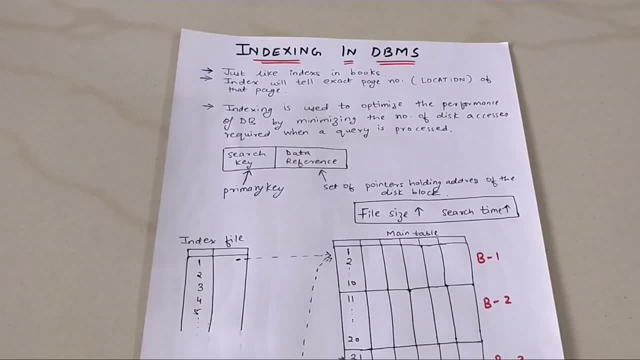 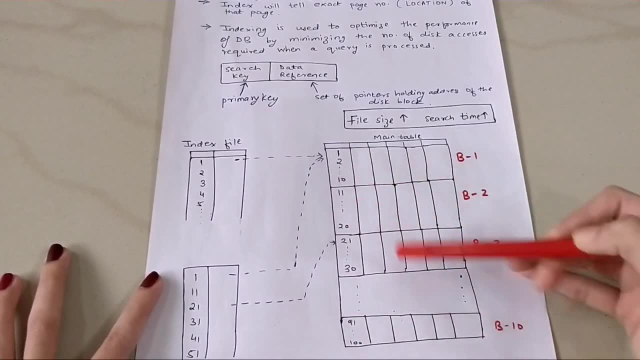 where the record for primary key one is stored. now you will ask me that this table is is having hundred rows and so many columns. whatever, this table is having hundred rows and so, and my index table is also having hundred rows only. so how is this table having hundred rows and so many columns? 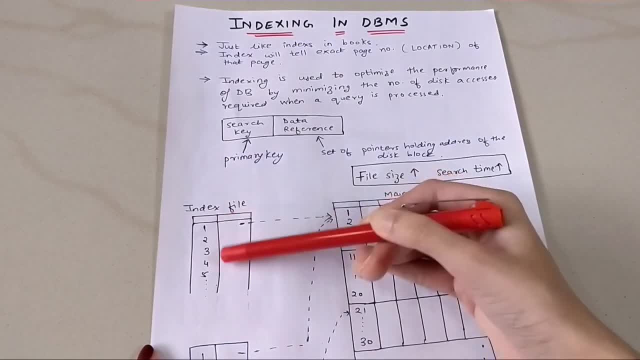 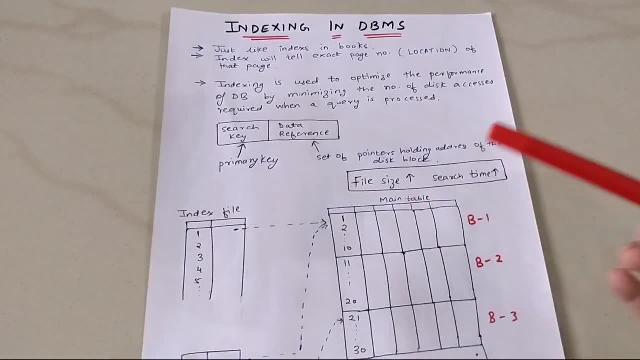 is it helping me? because i am checking this table as well. i'm checking this table before before finding out that particular record in the main table. how is it helping me? so you need to understand one basic thing: that the bigger the file size is, the search time will be more so for this table. the 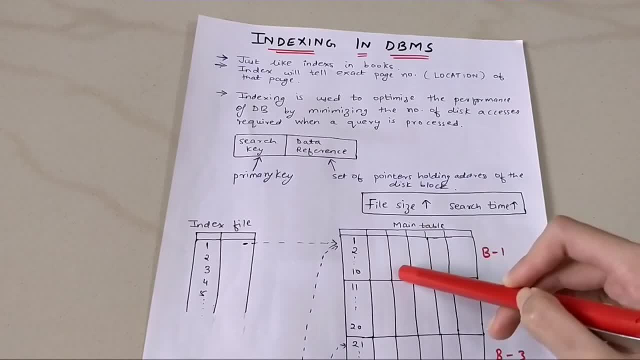 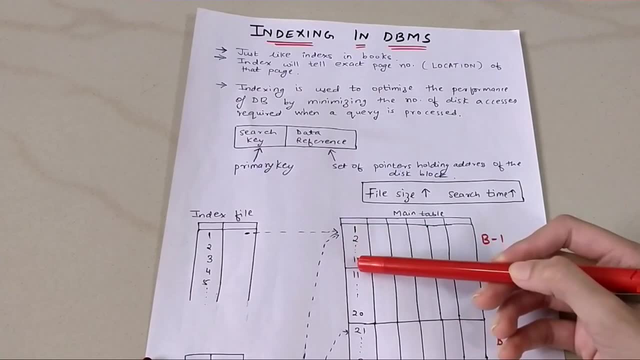 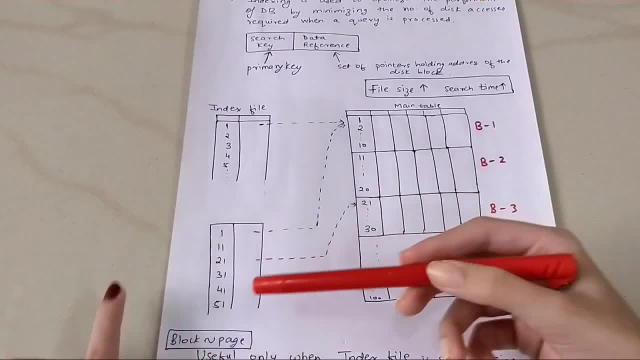 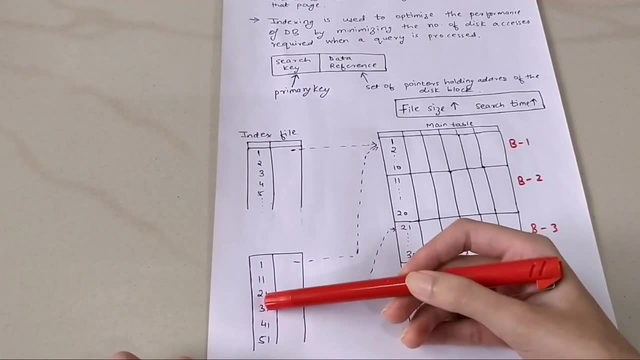 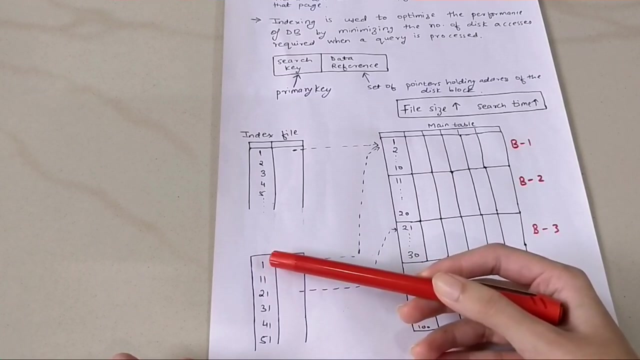 thirteen. so all of these are in ordered section. we can have another type of index, index file as well, index table as well, where we do not write all the records. so in this case, uh, i am only writing, uh, i'm only inserting the primary keys: one, eleven, twenty one, thirty one, forty one, fifty one, and these will 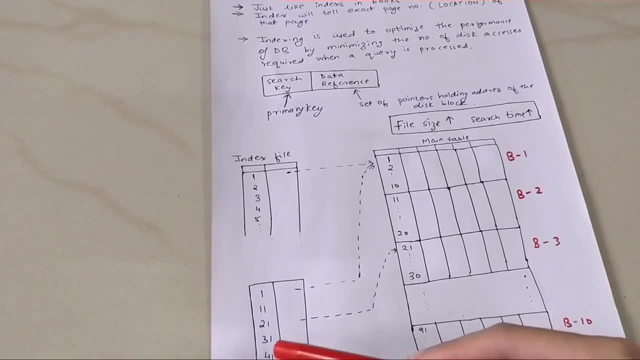 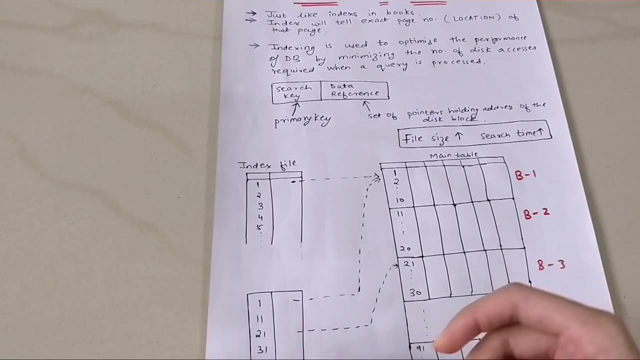 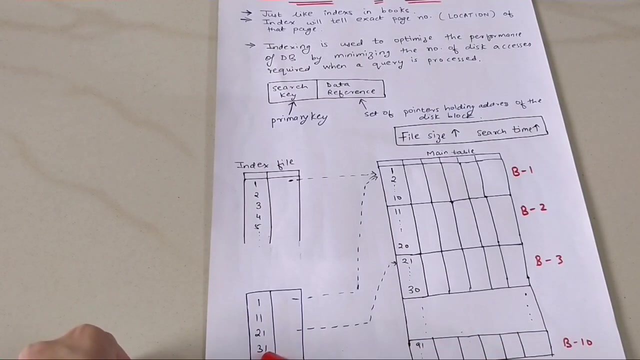 these will point to that particular block. now, if i ask this index index table to find find record 35 for me, so how will it find record 35 for me? it will, it will see where, where, it will check for index 31 and it will check where it points and it will go in that particular block and there it. 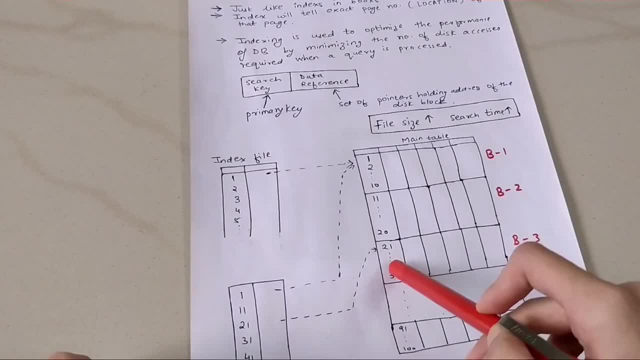 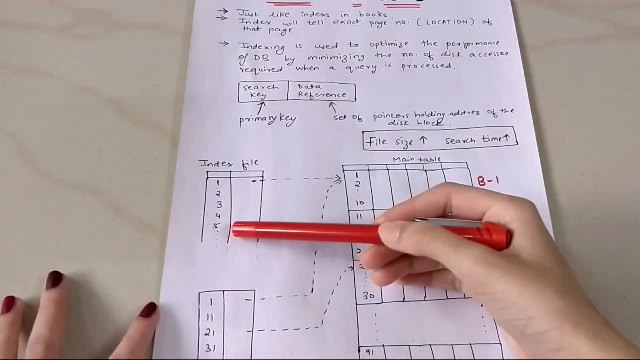 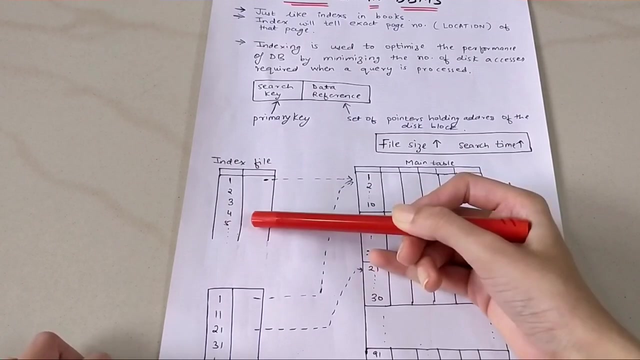 will find record number 35 and in this way it will help us in reducing the time to access a particular record. so the index index table where all the primary keys are written, all the primary keys are inserted, is known as dense indexing. okay, this is known as dense indexing, but in the detect stable. 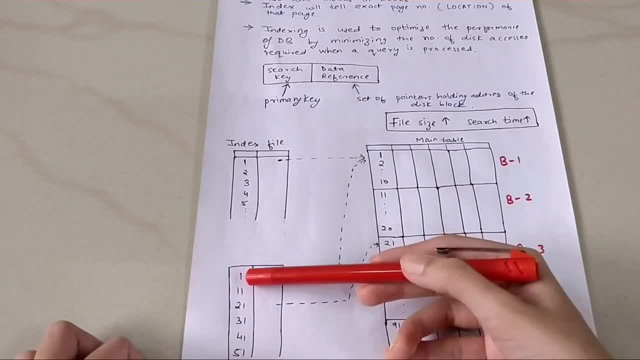 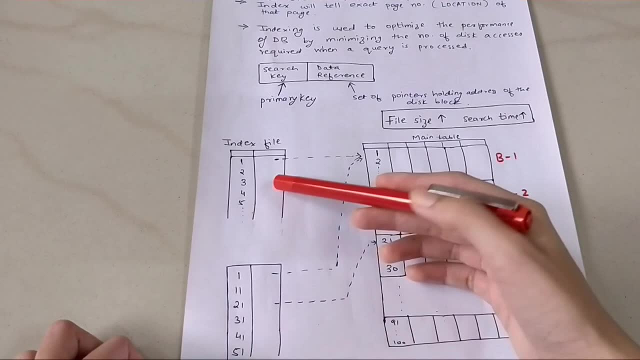 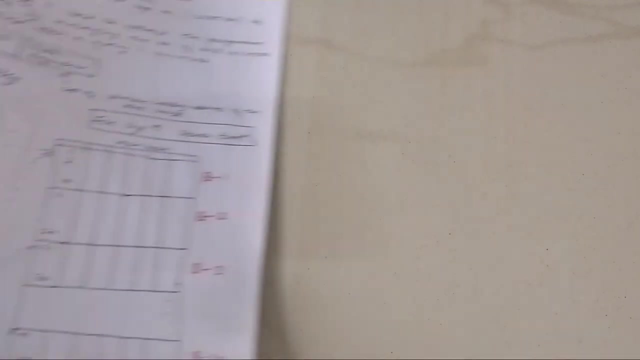 where all the records are not written but only specific records are inside, only specific primary keys are inserted, is known as places indexing. so these are the two types of indexing, and and the types of indexing will be discussed properly in another video. so so, in short, there are three Aires. 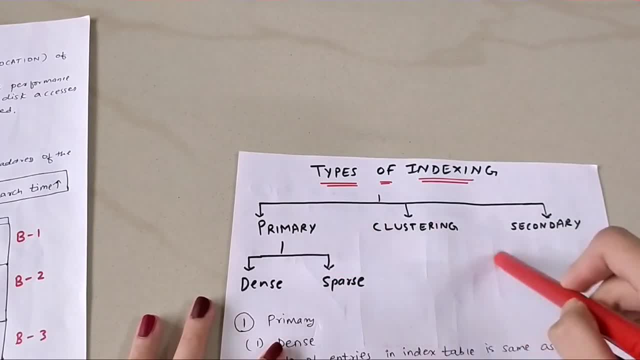 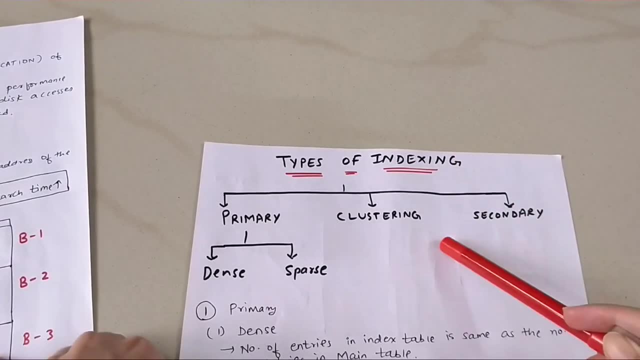 types of indexing: primary, clustering, secondary and then a Anna, even in India also- of indexing, so this will be discussed properly in another video. this is open夾y. so so in short, there are three types, and in primary we have densing spars and to understand or to learn about types of. 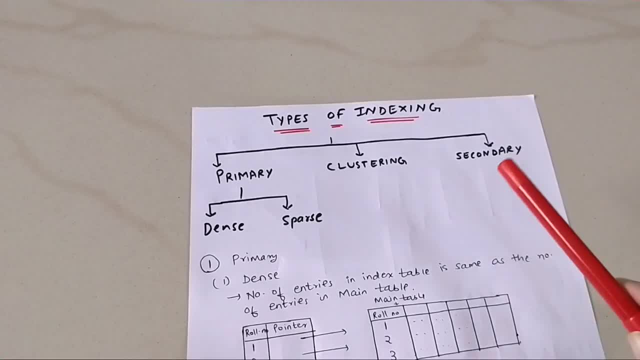 indexing. I will put another video soon. if the video is already uploaded when you're watching it, you will find the link in the description box. so please do check out the description box for the link of this video. so thank you for watching this video. 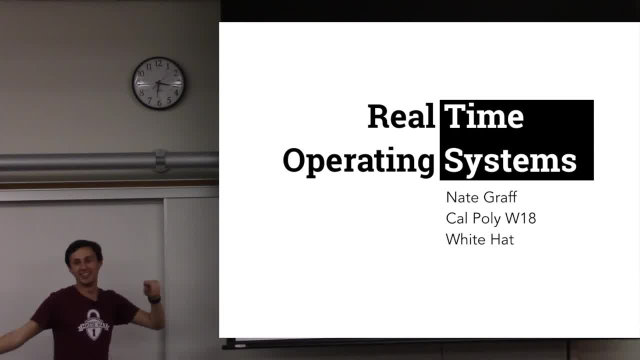 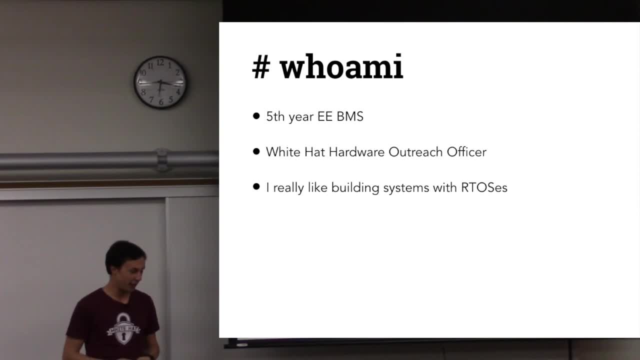 Hi everyone, I'm here to tell you about real operating time systems. So I'm Nate Graff, I'm a fifth-year EE blended master's student, I'm the hardware outreach officer for White Hat And I really like building systems with RTOSs. So when we